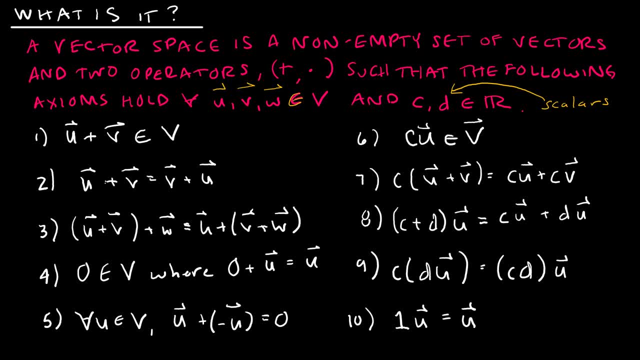 So, as we go through the axioms, you'll say, okay, I know that one, Yes, we've done this one, Yes, we've done this one. But what we've done up to this point is simply use them for. 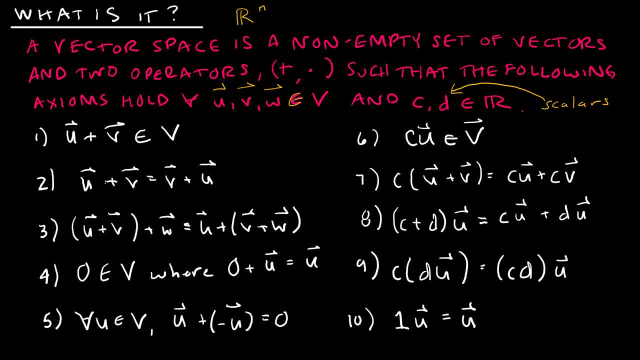 The set of Rn. So Rn is a vector space and all of these axioms hold true, which is why all of these will look familiar to you. It's because we've been here. We've been typically in R2 or R3, sometimes in R4 or R5, etc. 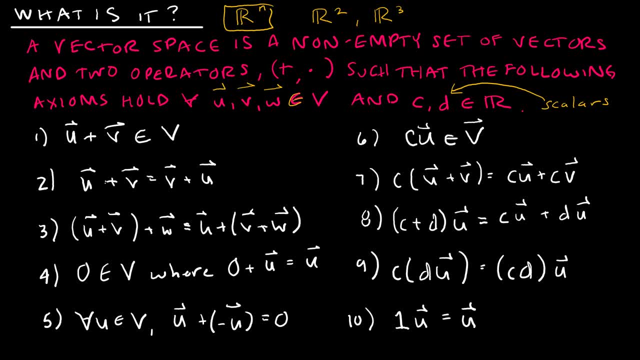 But what we want to do now is look at different spaces, and we need to verify these axioms to see if Those other spaces may in fact be vector spaces or not. So let's take a look at the axioms and try to make some sense of them. 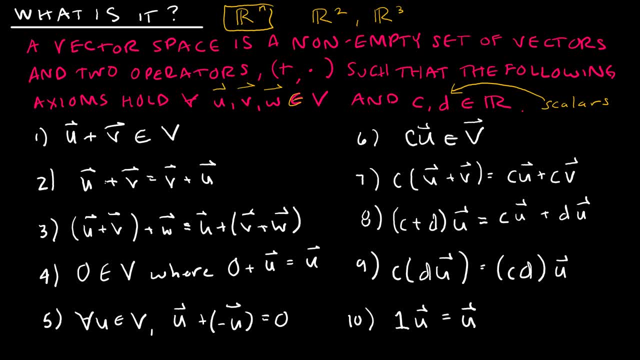 The first one simply says that if you have two vectors, then the sum of those vectors should also be in the set V. So of course this holds true for R2 and R3.. And again we're going to look at some examples where that might not hold true. 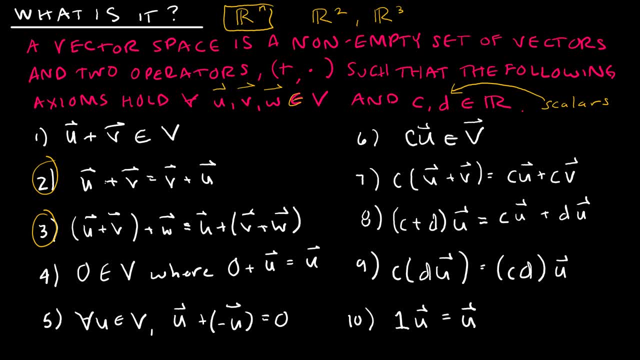 It also shows that. It also shows that It also shows that the associative and commutative properties- so commutative here, associative property here that doesn't look like an A associative property here- hold true. for addition, It also says that the zero vector. 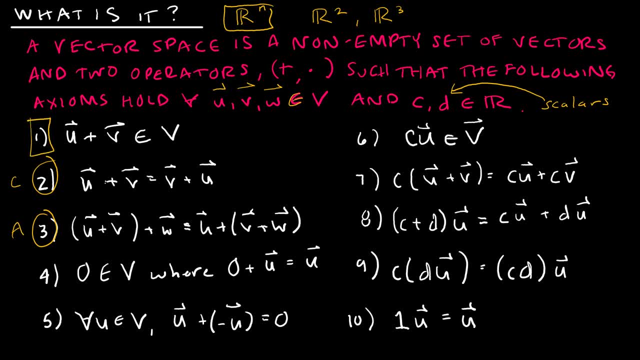 So I'm going to put a box around this one, and you'll see why in a little bit. It also says that the zero vector needs to be in our vector set or our vector space. where zero, The zero vector plus any vector, is equal to that vector. 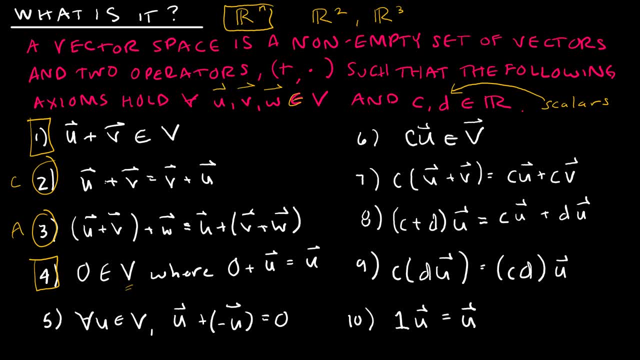 So this is essentially the identity And this is the inverse, The inverse saying I can add something, And again, each inverse is unique, but I can add some inverse to an existing vector. Both are in the vector space And The sum of those two vectors is zero. 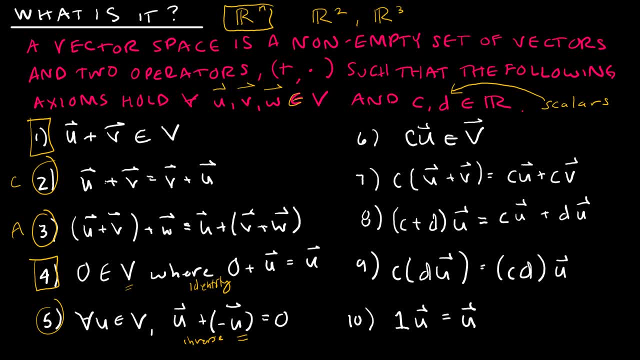 So those are all of the addition ones. Now let's take a look at multiplication. We again now have that a scalar times a vector is in the vector space, So I can take the scalar times something Whoops. 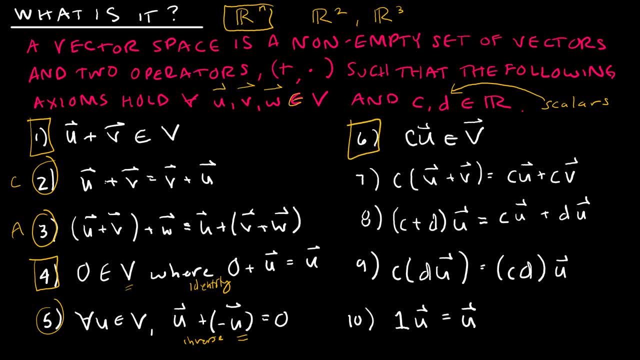 I'm going to put a box around that one, And then we have the distributive property that I can distribute, a scalar, that- And this is similar to the distributive property, Again just on the right side instead of the left side, but it's still distributive property. 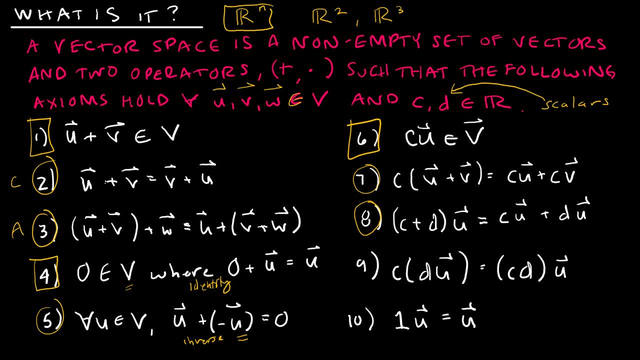 This one is the associative property And again it's associative with the scalars. So it's not associative. We know that matrix or vector multiplication is not associative or commutative, But of course, if we're dealing with scalars, those are: 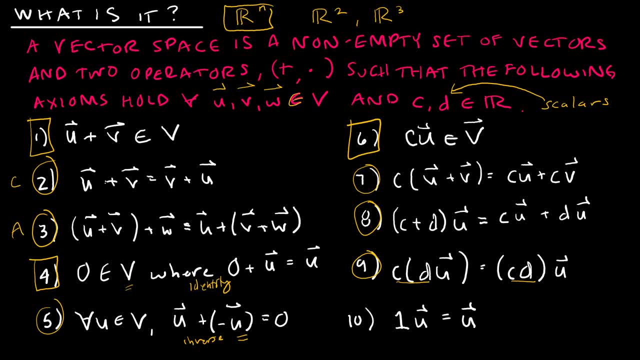 And then, back here again, we're down to the identity. So, as you can see, I've put a box around a few of these, And I've put the box around them because those are the ones that we will most often find issues with. 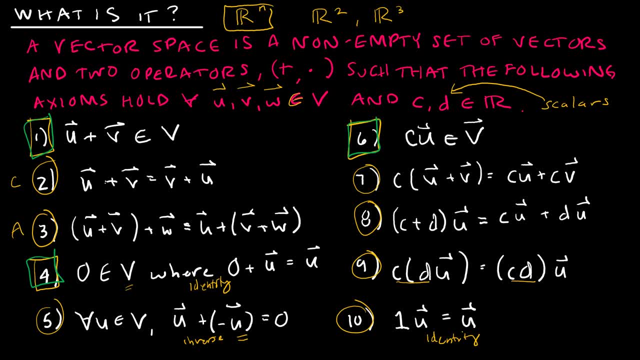 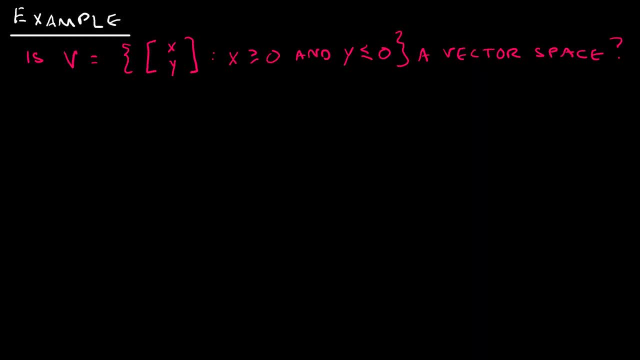 So those are the ones that you're probably going to want to check first. So let's take a look at a few examples of where we might not have a vector space. Let's take a look at an example which may or may not be a vector space. 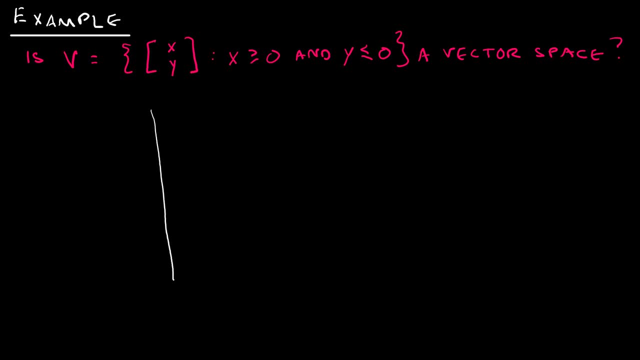 And I purposely started with some examples that we could visualize. As I said, we're going to get more and more abstract, So the examples that we'll be able to visualize will be fewer and further between. But here's a great example we can visualize: 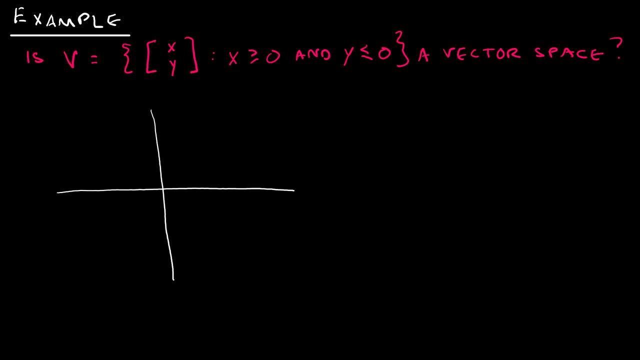 I have set V of all of the vectors- x, y, such that x is greater than or equal to 0 and y is less than or equal to 0. So I know, because I've been graphing for quite some time, that if x is greater than or equal to 0 and y is less than or equal to 0,. 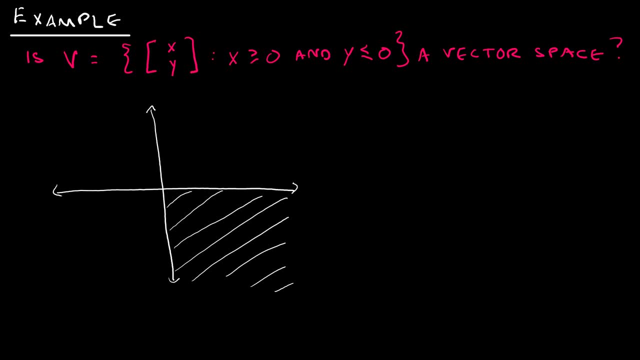 that's this space down here. That's the fourth quadrant. So my question is: if I have a vector in the fourth quadrant, will it meet all 10 axioms and in fact be a vector space? So let's take a look at an example. 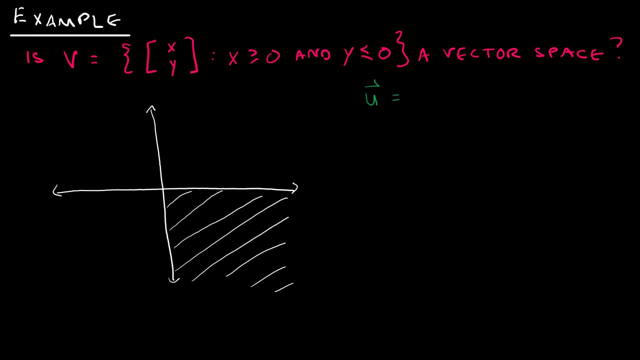 Let's say vector u is threeoops. I almost wrote that as an ordered pair: 3, negative, 1.. So 1, 2, 3, negative 1.. Here's vector u. Thinking about those 10 axioms. 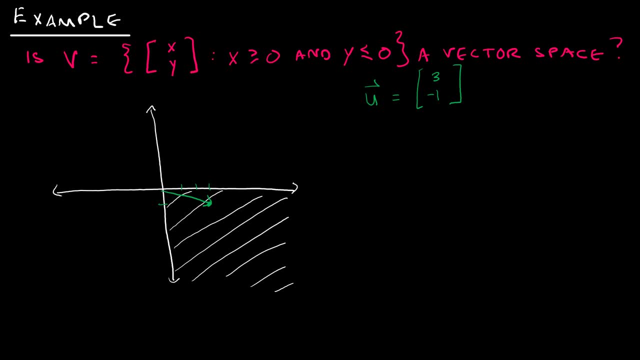 and there were three that I said were kind of the most important to check or the ones that you would check most often, where things wouldn't necessarily work out in your favor. let's start by looking at axiom 1,, which says the sum of u and v is in v. 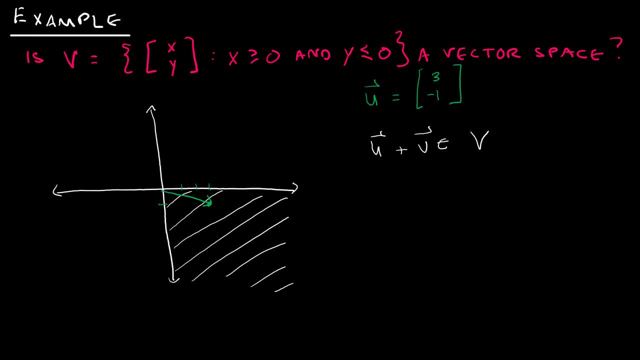 So I only have u. but let's take v. and obviously u is in v already, but let's give myself a vector v to just see. So vector v, let's say, is 1, negative 4.. 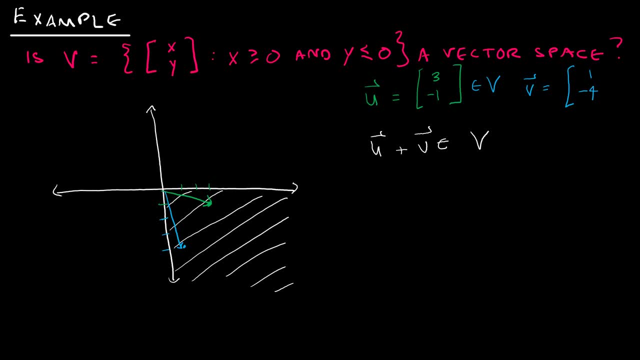 And again, this is also in v and I can see that because x is greater than or equal to 0, and y is less than or equal to 0, so I wouldn't have to have the picture to show that they are in v. 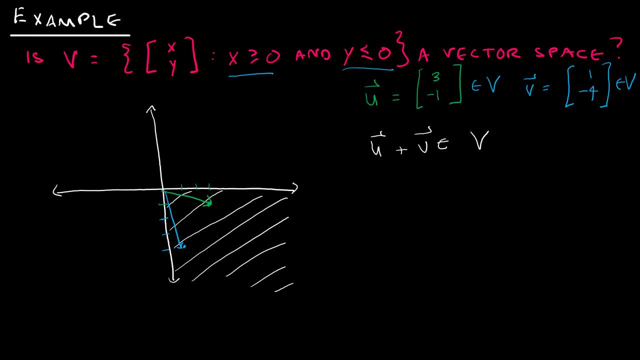 But my question is: is the sum of those also in v? So let's just see. Well, we know the parallelogram rule says So. visually I can just look at this and say, yes, that was a really bad parallelogram. 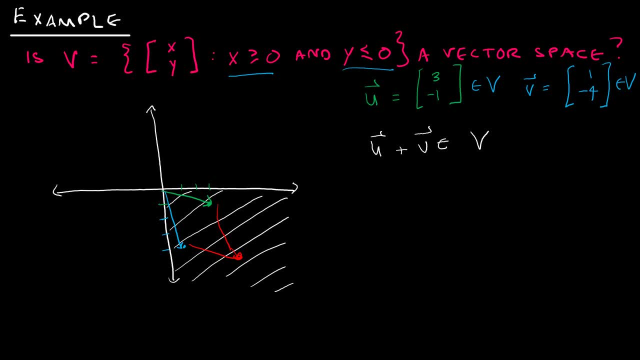 but you get the idea. But I can also add u plus v, which would give me 3 plus 1, or 4, and negative 1 plus negative 4, which is negative 5, and 4, negative 5 is in fact in v. 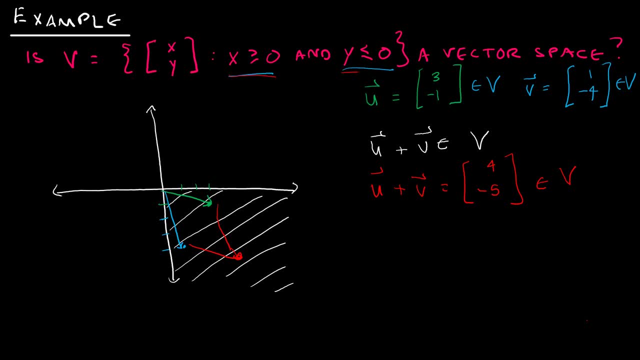 because x is greater than or equal to 0, and y is less than or equal to 0. So this one's okay. What's the next one? I said to check Number 6.. Just kidding, number 4.. Number 4 that says that the 0 vector is in v. 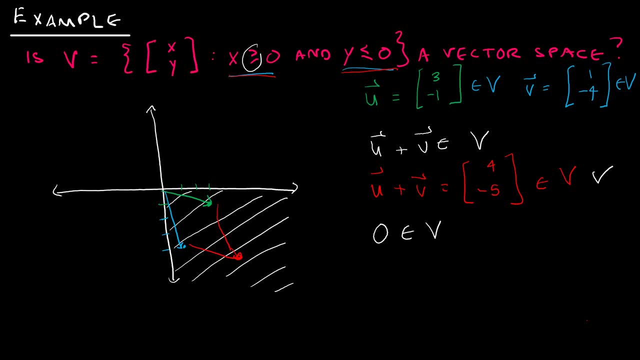 So, looking here, this is or equal to 0, or equal to 0,, so that means the 0 vector is in fact in v And the last one, which is 6, which says cu or cv. 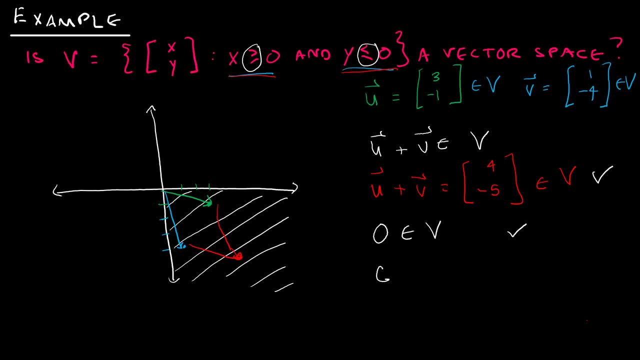 I don't remember which letter I used. Hey, quit changing colors on me. Cv is also in v. And keep in mind that c is just some real number, any real number that I want, And this one, hopefully, you can see. 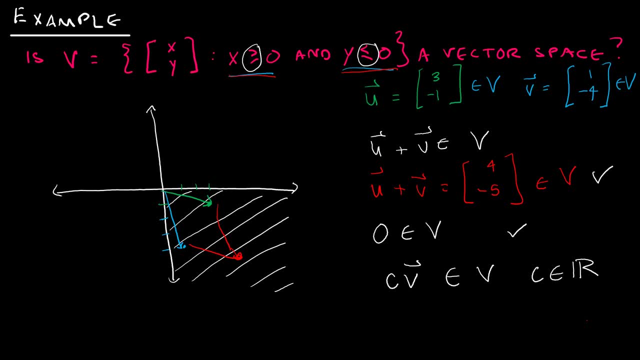 is just some real number. Hopefully you can see it's going to be a problem, Because what if c was negative 3? Then cv would be negative 3 times 3, negative 1, which gives me negative 9, 3,. 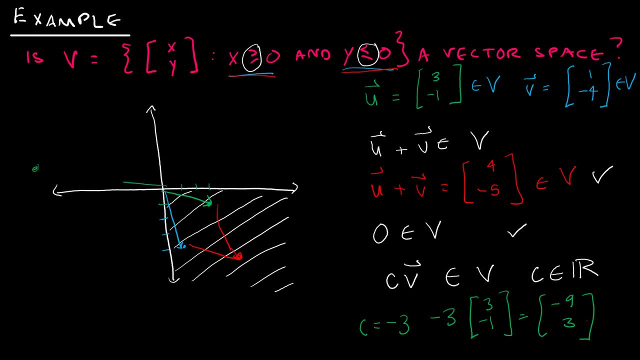 which is somewhere over here, which is clearly not in my region of x is greater than or equal to 0 and y is less than or equal to 0. So negative 3v does not belong to v and therefore this is not a vector space. 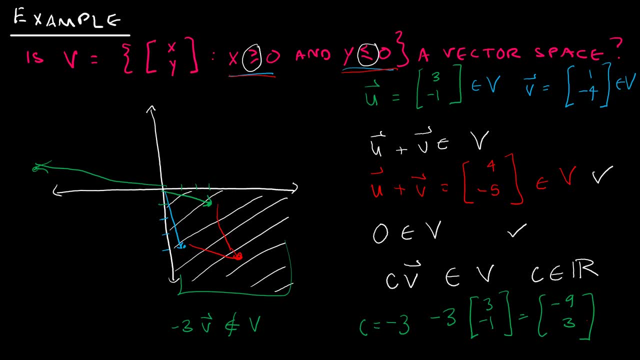 So notice I didn't say it doesn't meet axiom 6, because, remember, your professor doesn't have all the axiom numbers memorized. I have the concepts down. That's what you should do, too, is don't rely on those numbers. 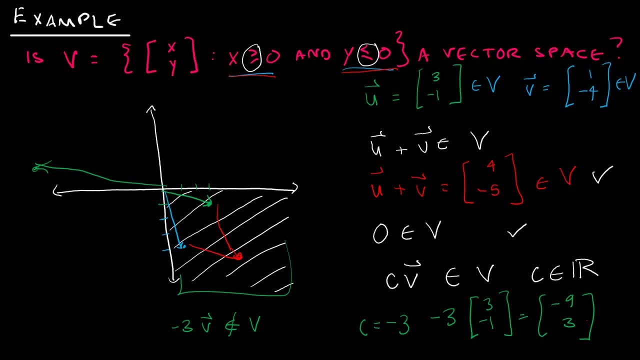 but rely on logic. So my logic says that I can't take all cv and have it belong to v. This one is not met and therefore it's not a vector space. Here's another practice for us that looks very similar. 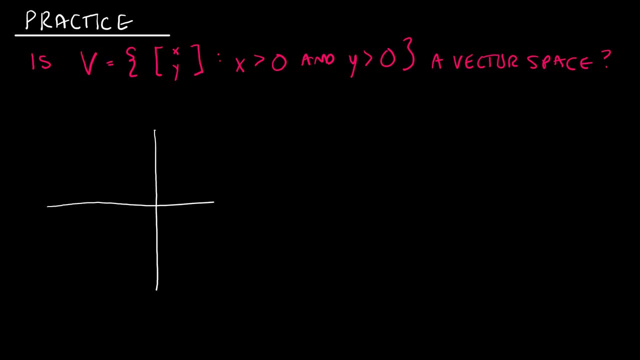 And, if you'll notice, the only thing I changed is I said that both are greater than 0. So you might be thinking: well, duh, Braim, we get it that this, in fact, will still be the case. 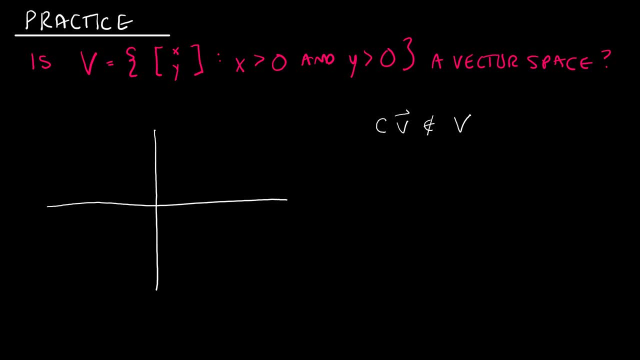 that I cannot take some vector that's in the space that I want where both are greater than 0. I can't take it times anything that I want and still end up in that same region, And that is true, But I wanted to give you this example specifically. 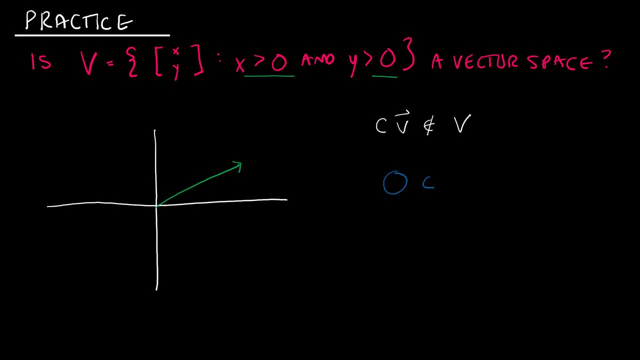 because this one also is that 0 is not the 0 vector, which is 0,. 0, is not in v, because this is greater than 0 and greater than 0, so 0 is not included. So again, obviously. 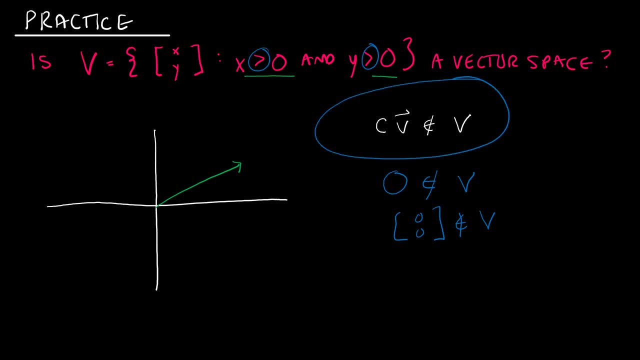 we already knew, based on this, that it was not going to be a vector space. but the fact that the 0 vector is not included also tells us that v is not a vector space. Here's a practice for you to try on your own. 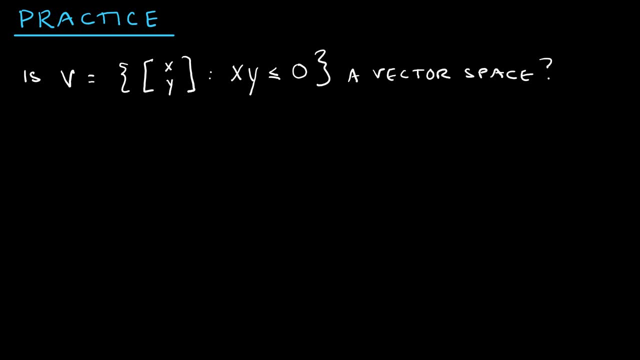 so give this one a try. When you're ready, press play to see how you did So. again, this is one that we can visualize and we are saying that x- y is less than or equal to 0, which means x- y is negative. 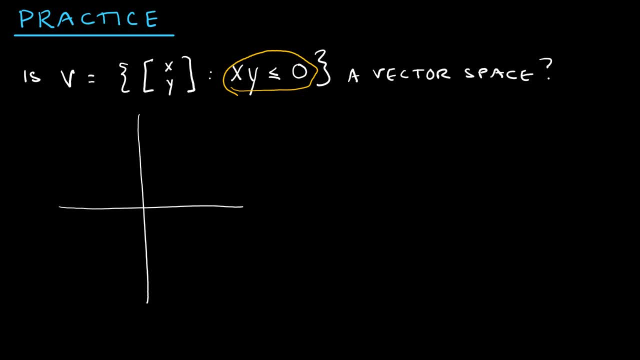 or equal to 0, and that would mean that either x is positive, y is negative, or x is negative, y is positive. So here's what we're dealing with. So let's check a couple of those axioms that have a tendency to give us a hard time. 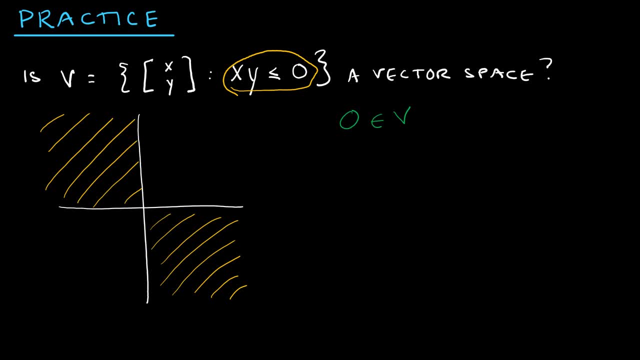 For instance, is the 0 vector in v? Well, because it's or equal to 0,. yes, in fact, that is true. I could have v as 0, 0,, which is the 0 vector. What about cv? 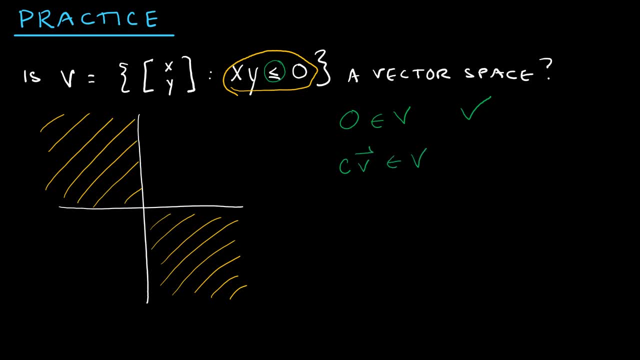 Is that in v as well? So quite often this is one that gives us a hard time. For instance, let's say this is 2, negative 3.. We'll say v is 2, negative 3.. This certainly is in v. 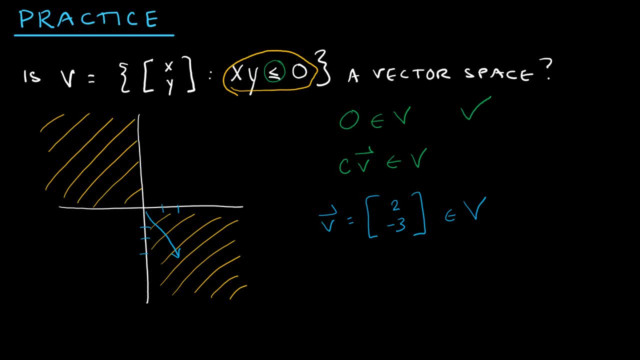 because 2 times negative 3 is negative 6, and that is less than or equal to 0.. And what if I took that times a positive value? Well, that would give me 6, negative 9,, which is still in that same region. 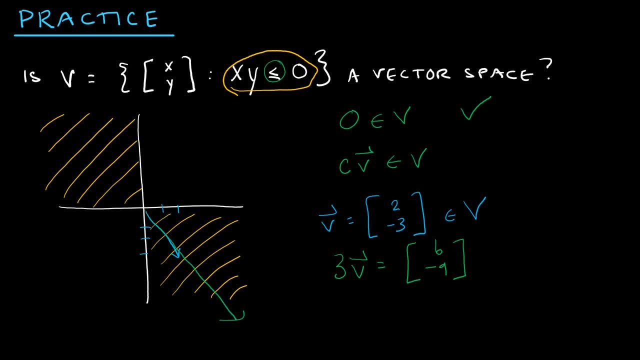 Okay, it's just going to make this guy longer. What if I took it times negative 3?? Well, that would give me negative 6, positive 9.. Would that still work? Well, if I multiply those two, that is still less than or equal to 0.. 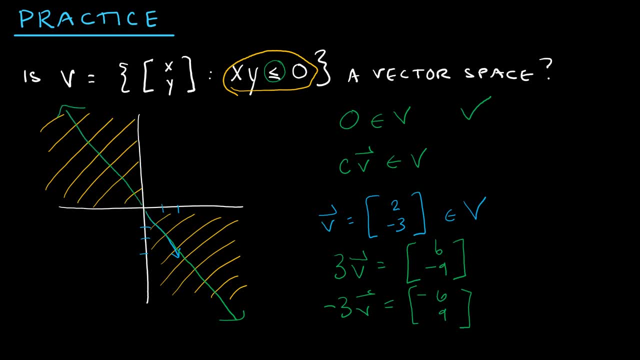 And in fact it would just be over here. And so, yes, we are just fine, This still holds true. So, check, check. I've got two checks. Now let's go back to that very, very first one. 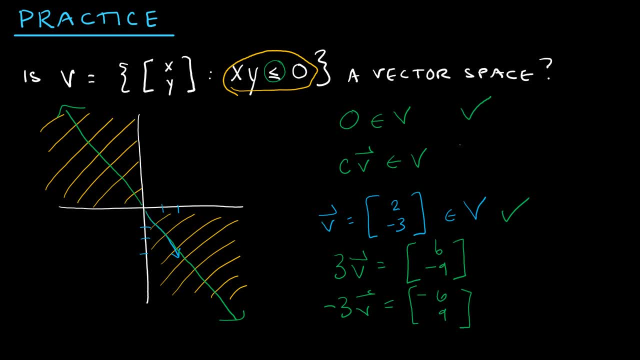 that says u plus v must be in v. Well, let's say I'm going to get rid of these green guys here. Let's say: that's my first one and we're going to make I'm going to get rid of this. 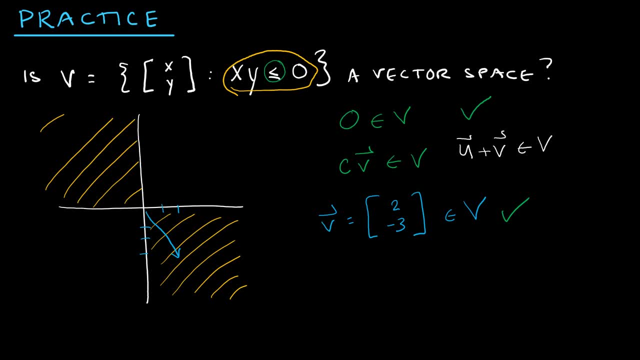 Running out of room here. So let's say that u is negative 1, 5.. So negative 1, 5. up here And again, what is then? u plus v? I would end up with 2 plus negative 1,. 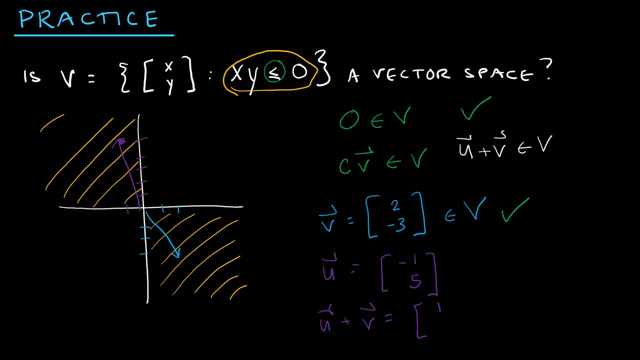 which is 1,, and negative 3 plus 5,, which is 2,, and 1, 2,, which again parallelogram rule. We could see clearly. this guy is not in v and therefore no. 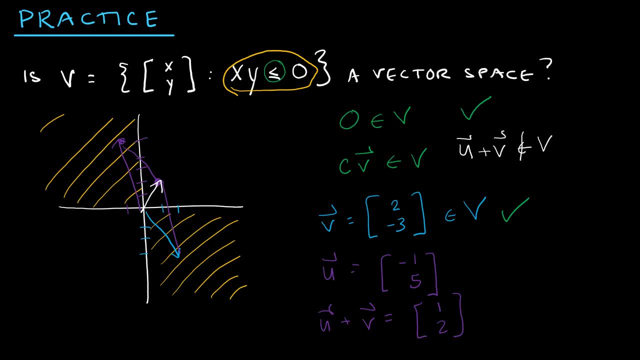 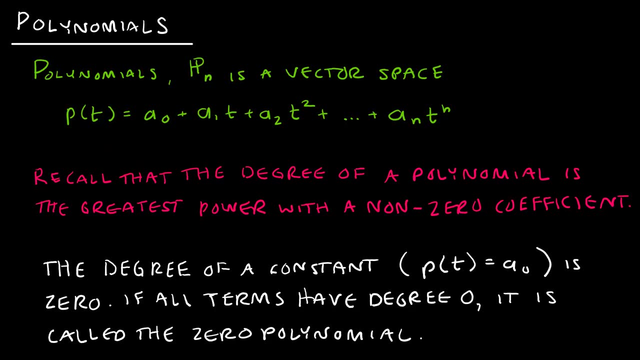 because this guy is not true. Therefore, this is not a vector space. Let's take a look at polynomials. Polynomials, in fact, is a vector space, which seems a little counterintuitive, but we can see in the way that this is written. 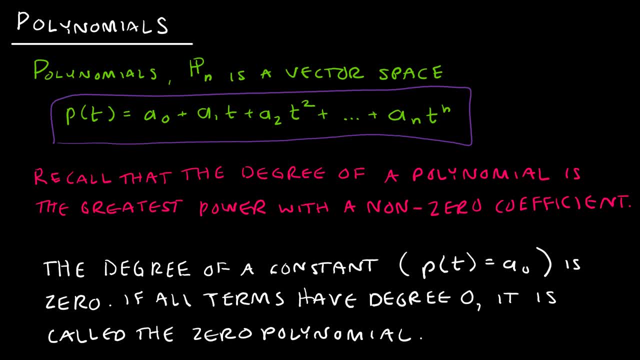 that it's written very much like a linear combination of scalars and vectors. Same idea, And remember that the degree of a polynomial is the greatest power with a nonzero coefficient. So in this example, n would be the degree of my polynomial. 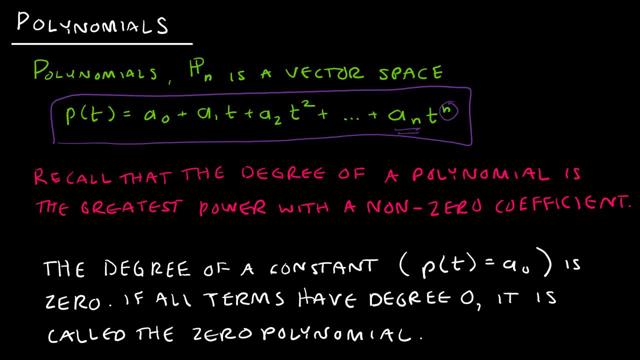 assuming that an is not 0. And the degree of a constant is 0.. So, for instance, if my polynomial- Oops, I went ahead and wrote it down here- So if my polynomial was just equals a sub 0,. 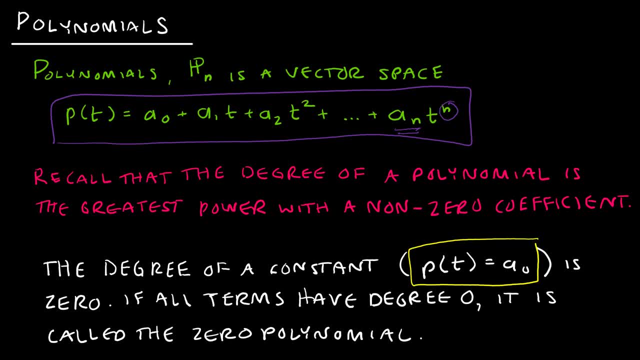 meaning I don't have a t or a t squared or a t to the n, then that is the 0 degree, And if all terms have degree 0, then obviously the highest degree would be 0, and that's called the 0 polynomial. 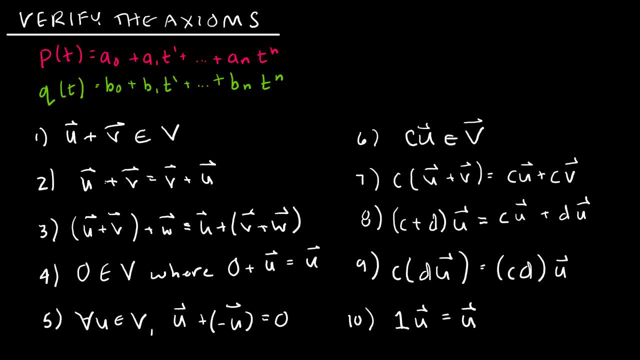 So let's verify the axioms to ensure that this is in fact a vector space. So I've listed the axioms here so that you don't have to have them memorized. But let's take a look at the first one. 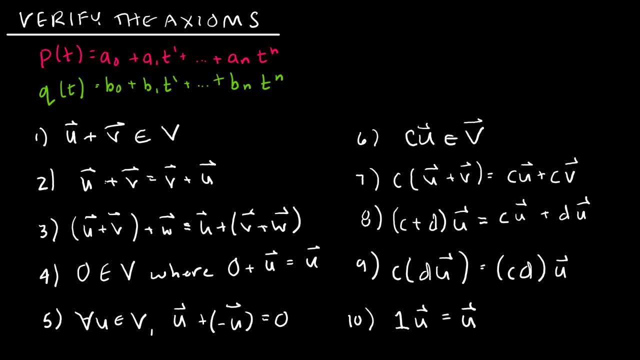 that u plus v would in fact be in the vector space. So we know the vector space essentially are terms that look like this: They're going to be a polynomial written in this form. So if I added, say, p and q together, 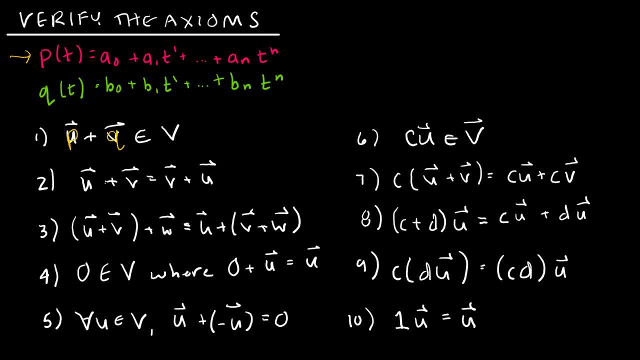 so I've written these in terms of vectors. but if I added p and q together, would it in fact be in that space? So if I take p of t plus q of t, what would I get? I would get a 0 plus b 0.. 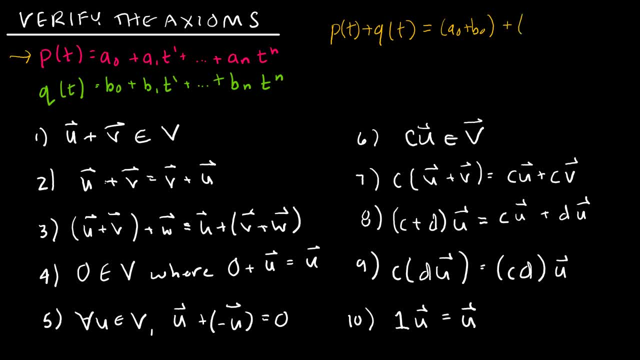 And then I would get a 1 plus b 1 t, because I'm adding like terms plus, et cetera, et cetera, And that pattern would continue. and would that in fact be a polynomial? Yes, I would just be combining those like terms. 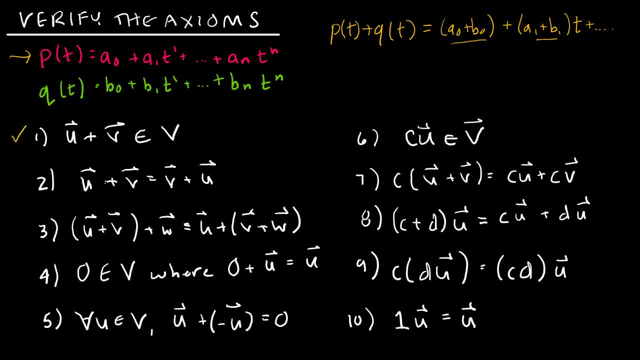 So this one does in fact hold. Now, what I know about real numbers is that addition of real numbers is commutative and also associative. So I'm not going to check those, because I know that if these guys were in the opposite order, 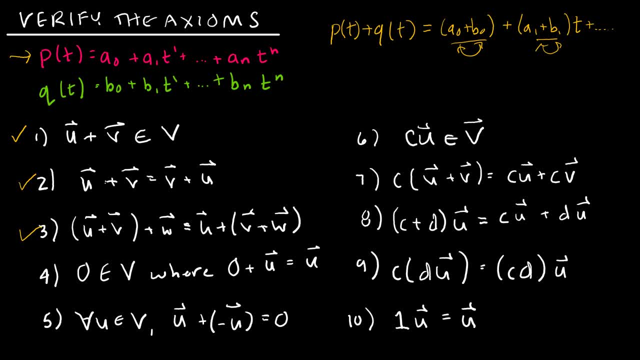 that would still be okay. And if I were grouping things differently? I'm still combining like terms and that's okay. So those have been checked and verified. Is the 0 vector? Well, that means oops p of t. 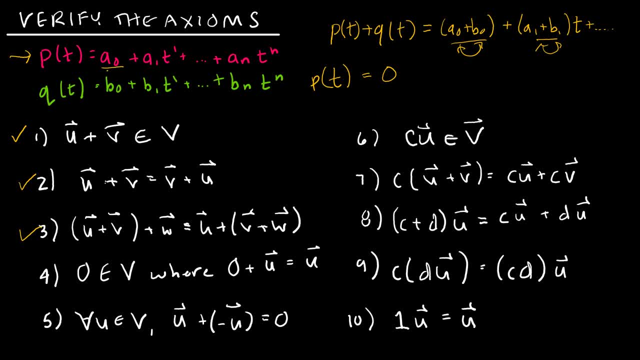 what if p of t were 0?? Would that fit this? Yes, that would just be that a of 0 was 0.. Is that in the space? Yes, it is, And if I added this to any other polynomial, would I end up with a polynomial. 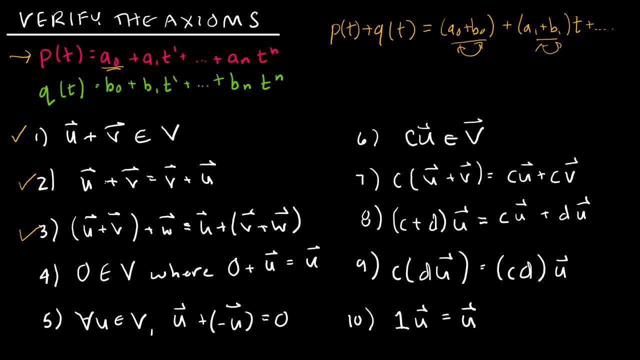 Yes, I would. What else can I check? Let's check the inverse. So p plus negative p. well, it would certainly make sense if I had a 0 and let's say q of t were negative, a 0, and then this was a 1 t.